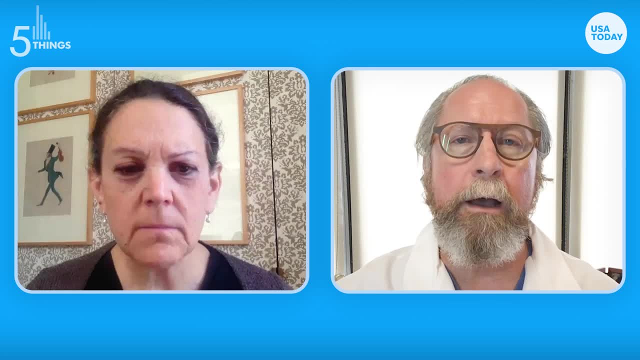 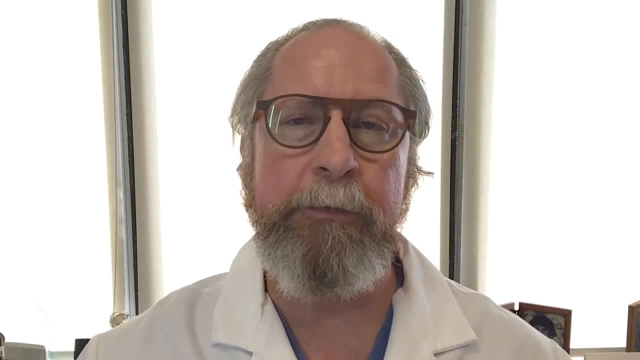 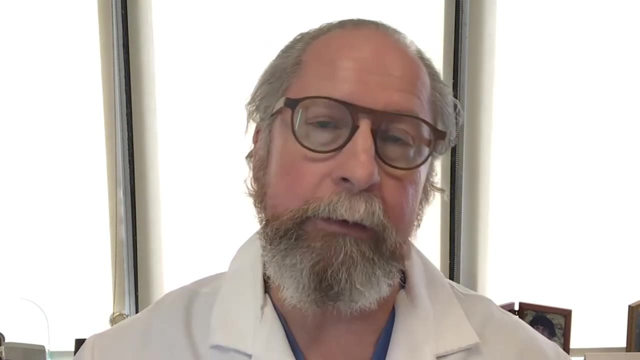 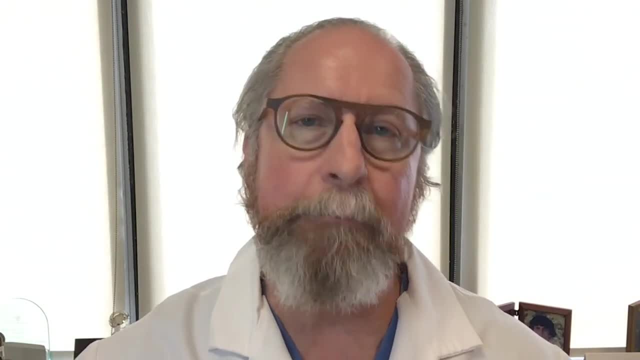 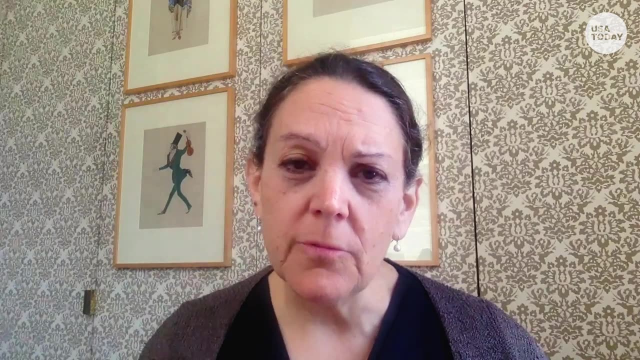 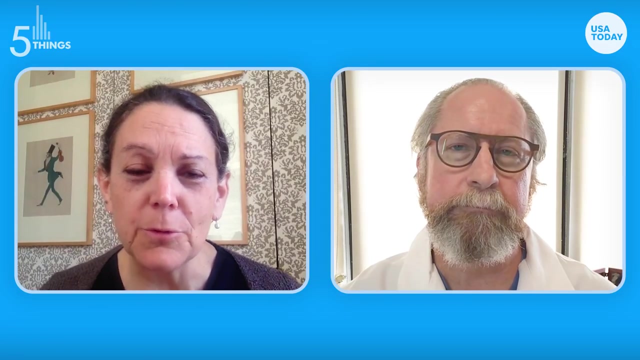 option where he could donate his entire body for the purposes of a research study. Mo's been in this ICU room for about two months. that had special meaning for you, and not just because it had a beautiful view of the East River. Can you explain a little bit about what that room? 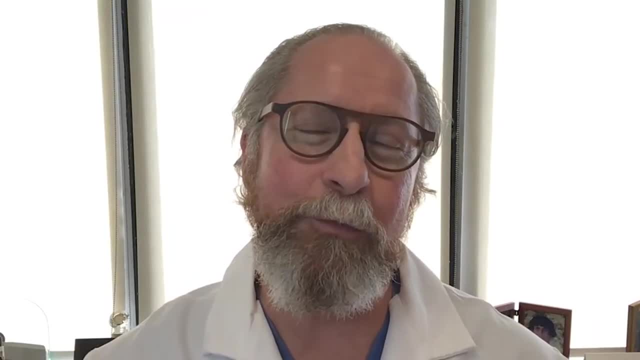 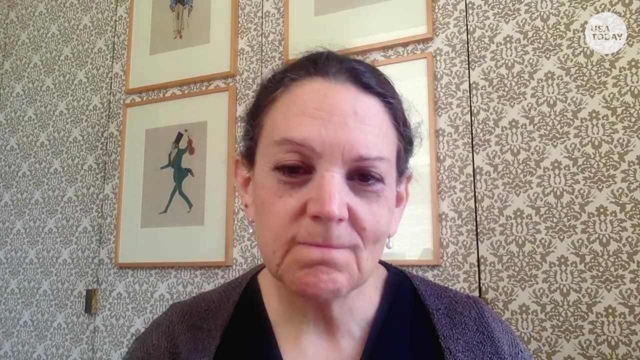 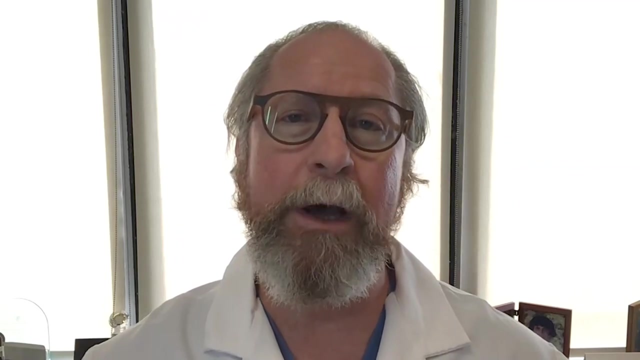 means to you, meant to you. The special significance that the room has is that's where I spent over a month waiting for a heart transplant five years ago- almost exactly five years- and then recovering from that transplant, And that's where he spent two months with a. 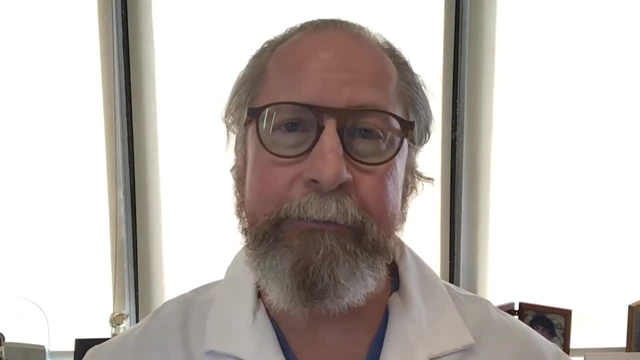 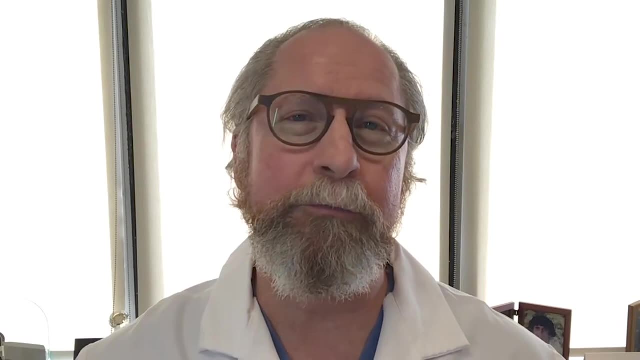 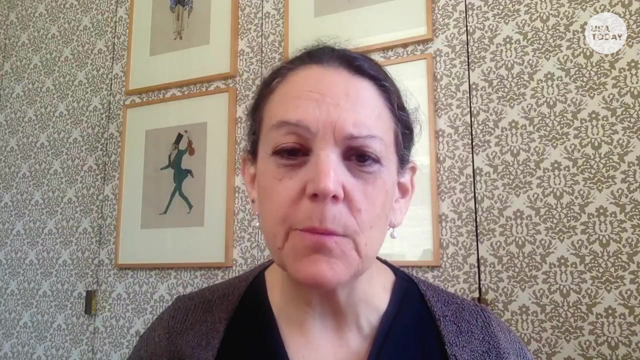 heart transplant And that's where he spent two months with a heart transplant Pig kidney inside his body, doing everything that was required of it to filter out the toxins in his blood and do all the other things that a kidney does. Why did Mo or his sister agree to let him? 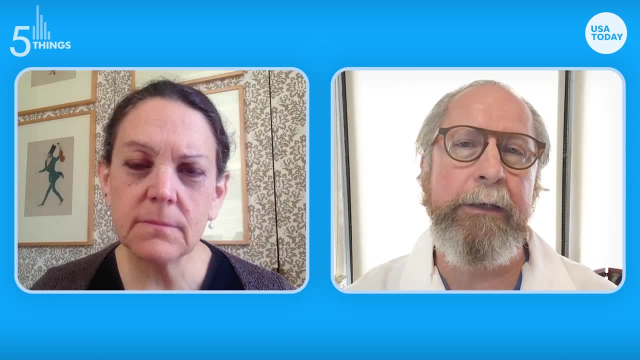 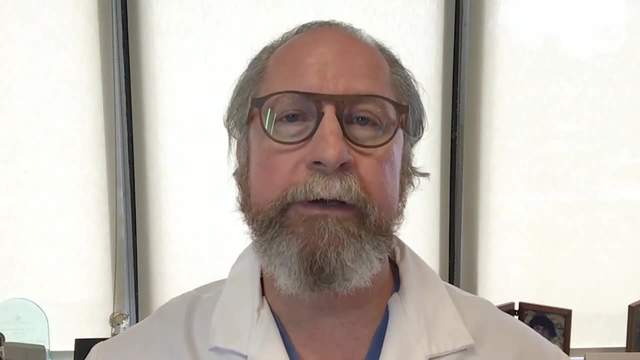 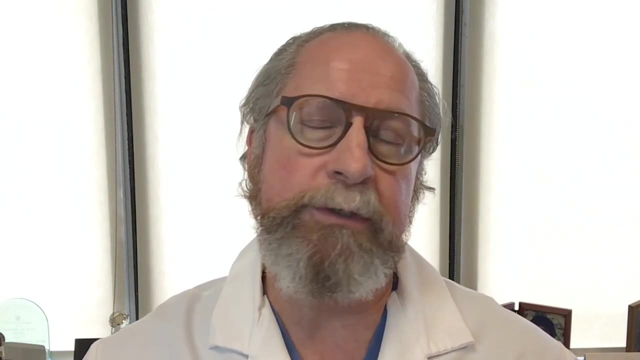 participate in this research. Mo's sister, Mary, who was very close to him, really felt that this was something that he would want. He was a very kind-hearted person. He was a very kind-hearted person, very giving, cared about other people, And so she thought this was in perfect alignment. 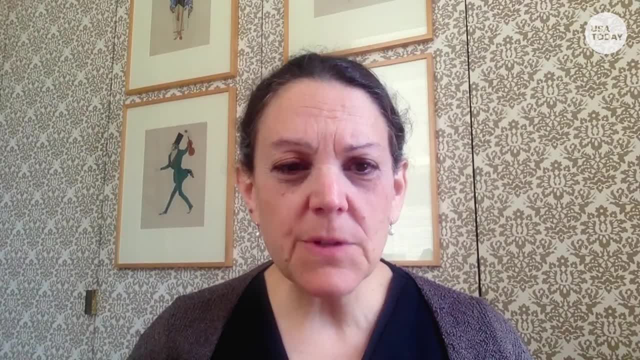 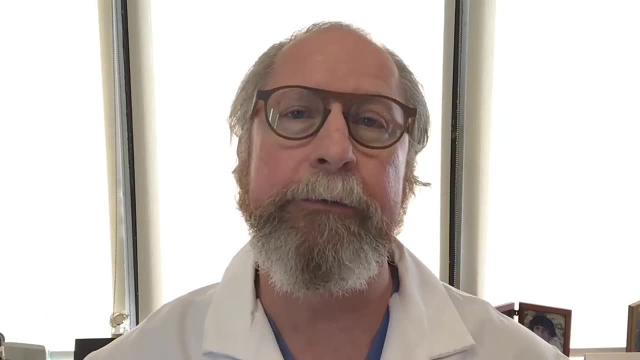 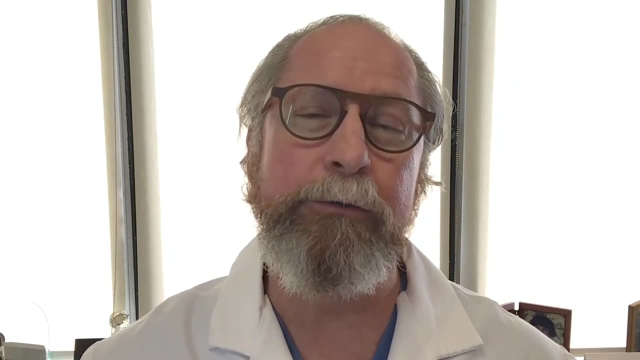 with the person that he was And talk to us a little bit about the surgery, the process itself. What did you do? We set up the transplant just like we would any other transplant between two humans. So we sent a team down to Virginia where the pig farm is on a jet. 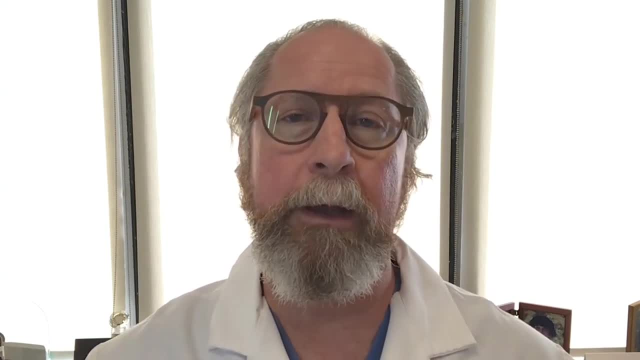 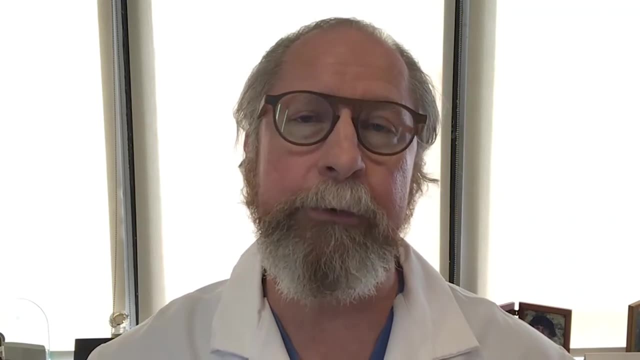 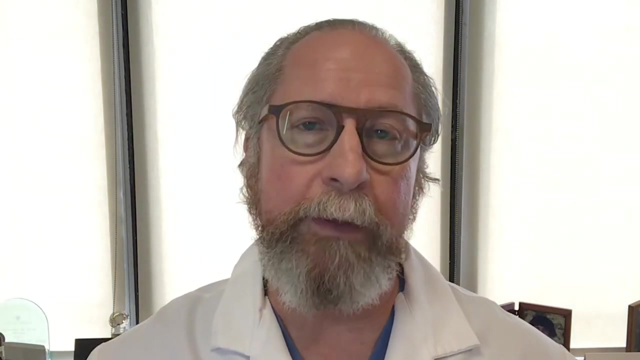 And they procured the pig's kidney and flew back. And at the same time I started the recipient operation on Mo And we did the kidney transplant just like we would a regular transplant, except for one thing: We removed his own kidneys, so his native kidneys. 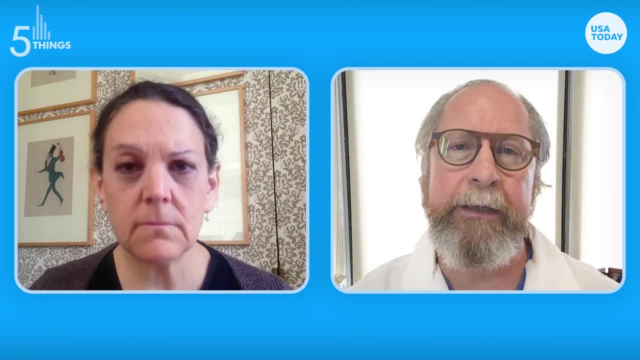 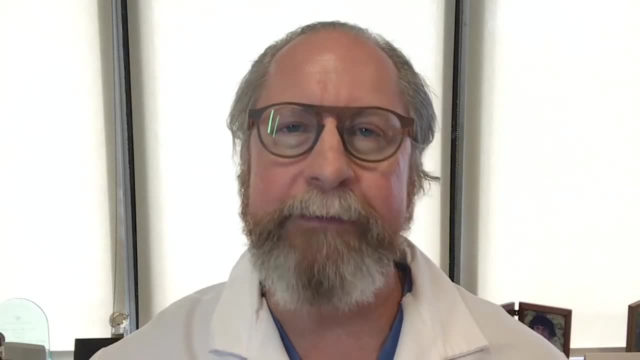 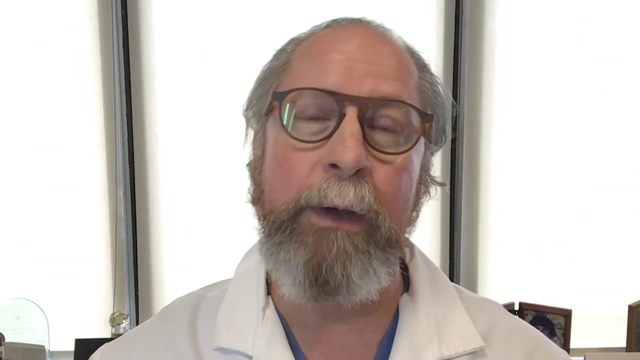 so that all the urine and all the work that a kidney has to do would need to be done by the gene editor Pig kidney. So we would be able to separate that out and really test the kidney and know exactly what it was doing and how well it was performing. Can you tell us a little bit about the pig? 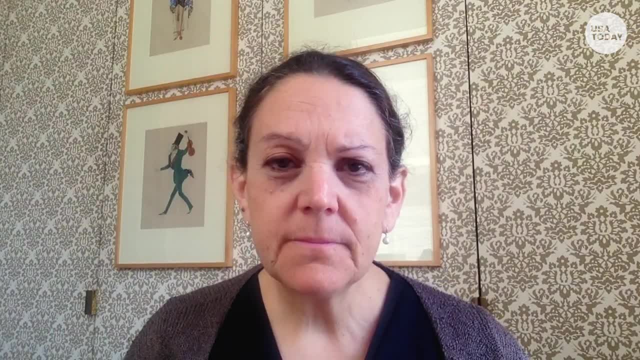 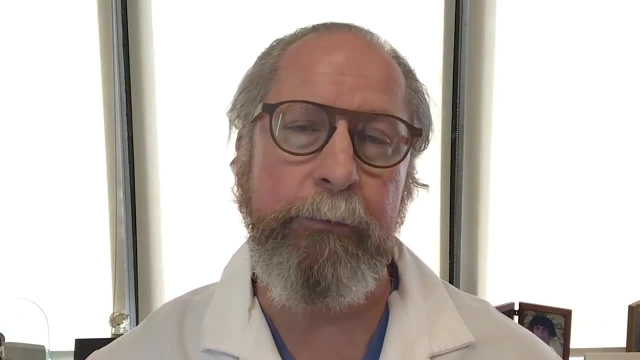 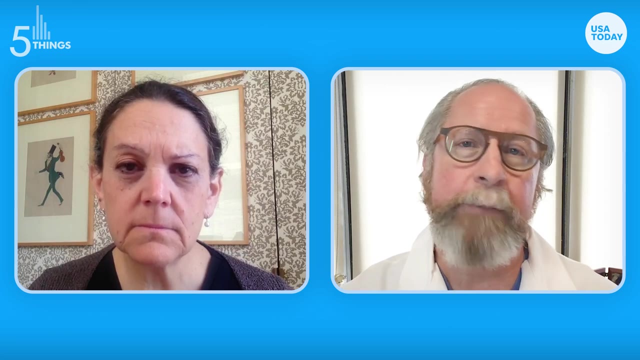 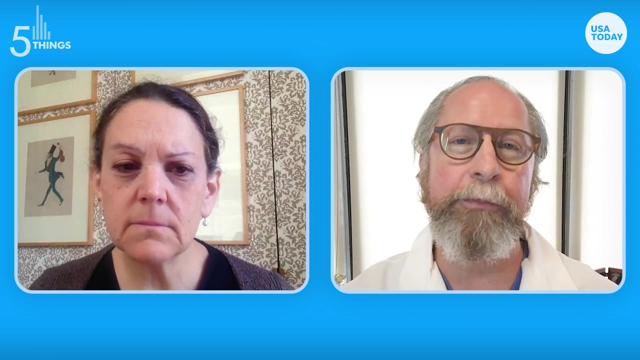 gave its life. for this procedure, The pig is raised in a very clean environment and is monitored. We do surveillance for about 35 different pathogens- viruses, bacteria, parasites- And so we know exactly what the state of that pig's health is and exactly what it's. 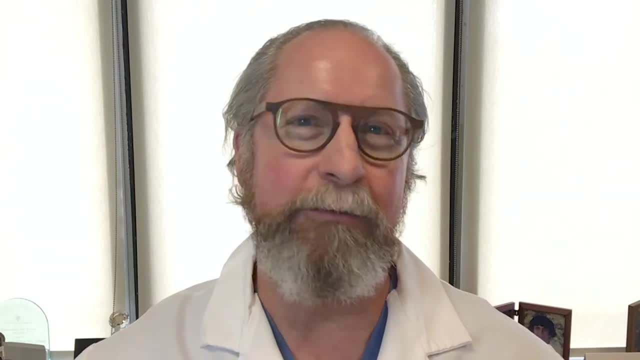 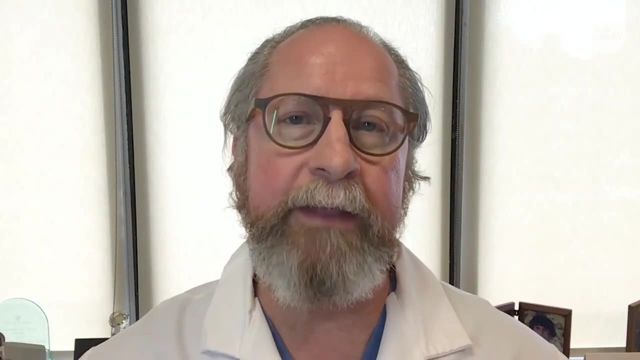 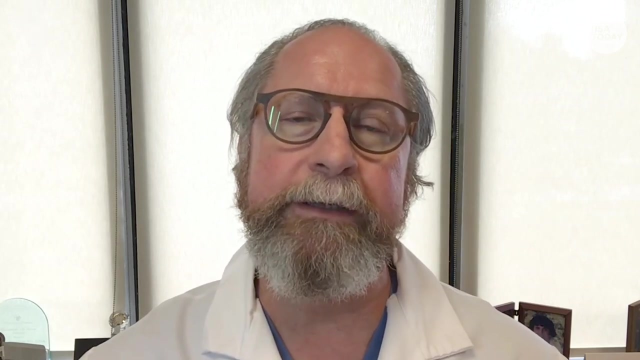 been exposed to. It has a lot of activities and toys and things like that. And then at the time that we remove the kidney, it's given a general anesthetic so it doesn't have any pain, And then given a lethal injection after the kidney is removed, And then we have a lot of 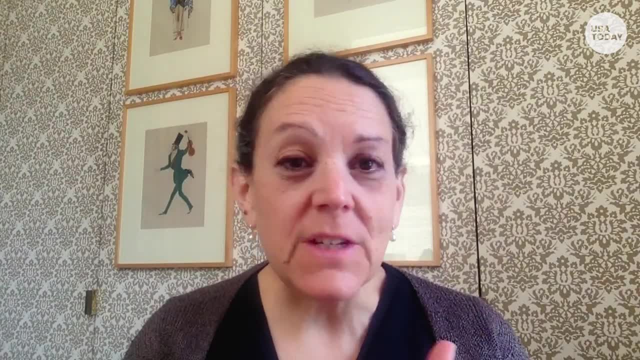 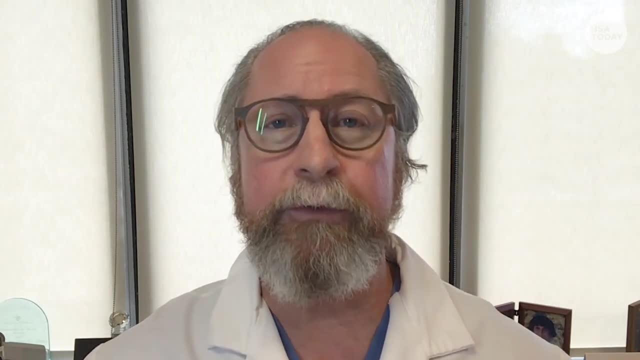 tests to do to make sure that the kidneys are removed? You talked about the gene editing. What genes are edited in this pig? So for this particular pig it's actually a pig line. So there's a herd of pigs, They're called gal safe pigs And they've had one gene knockout And 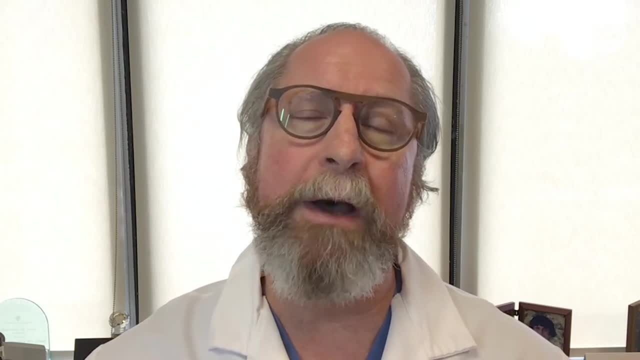 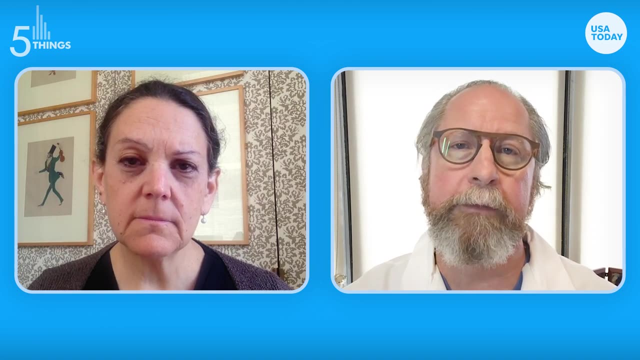 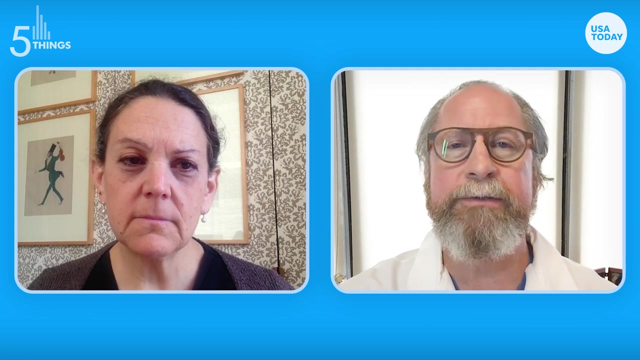 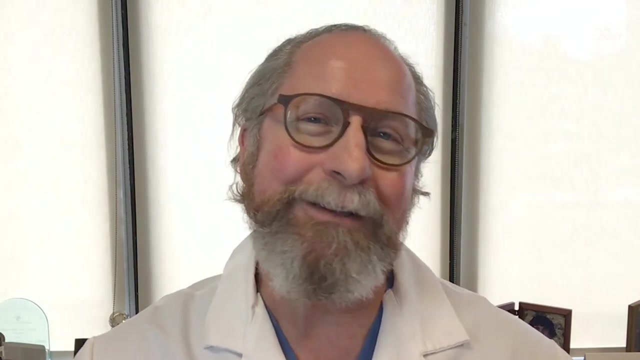 that gene is responsible for creating a carbohydrate that coats all of the cells of the pig And that carbohydrate- the enzyme that makes that- has actually been lost during evolution from pig to human. So humans don't express that carbohydrate, but that carbohydrate is shared by bacteria, So we make. 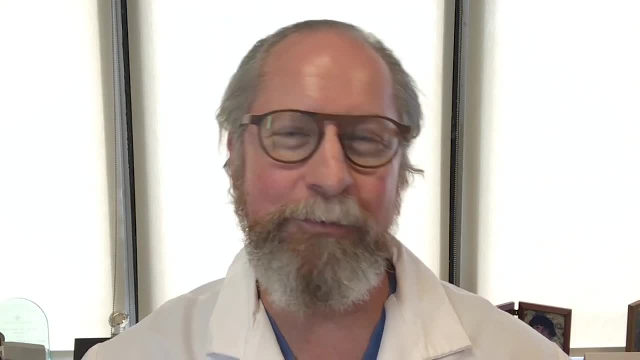 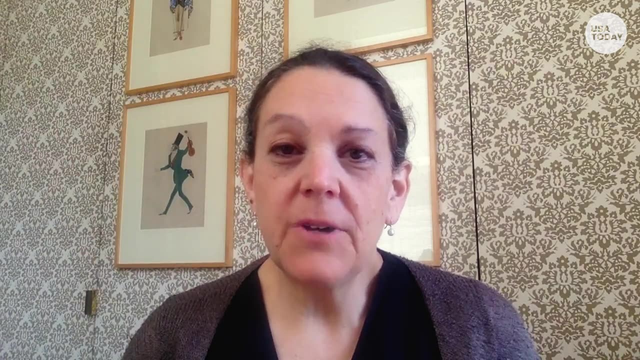 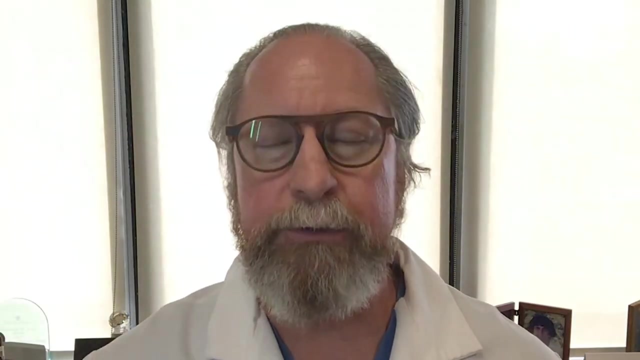 a very strong immune response to that carbohydrate in order to keep bacteria inside our gut. So the purpose of this research was to see if the kidney could function. the pig kidney could function in the person without triggering an immune response. Dr Howard Bauchner, It wasn't rejected and had a good function. 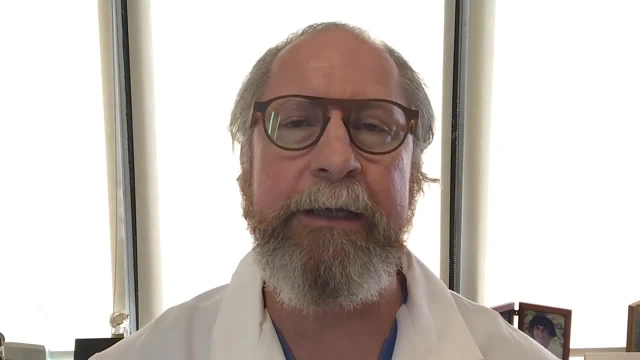 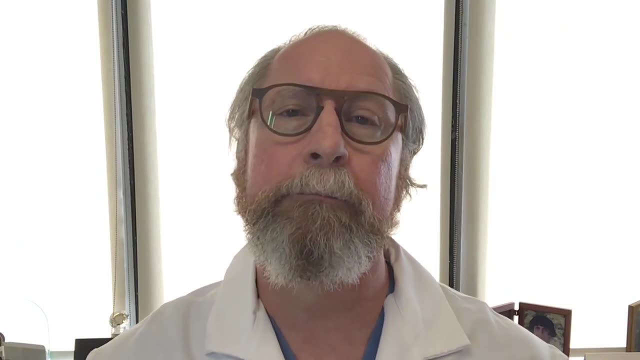 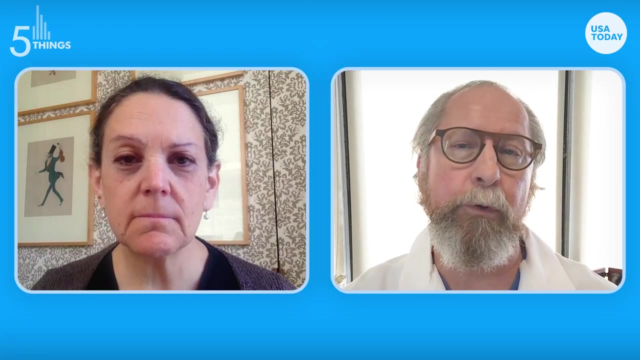 but that's about all we could really answer from a three-day study. For this longer study, which in the end we re-approached the family and our institutional review board, We got permission to extend it to two months and we were able to answer some important questions. Number one: 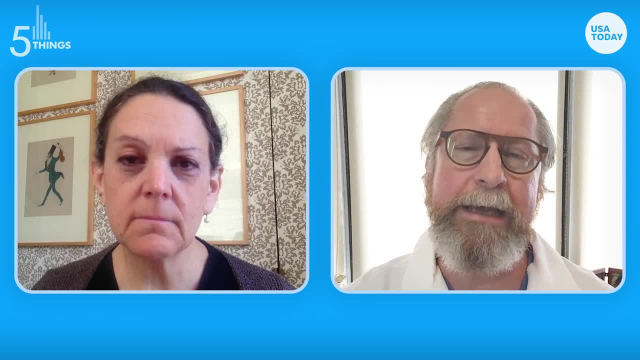 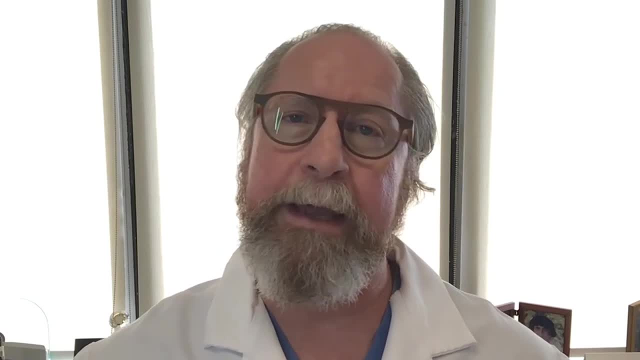 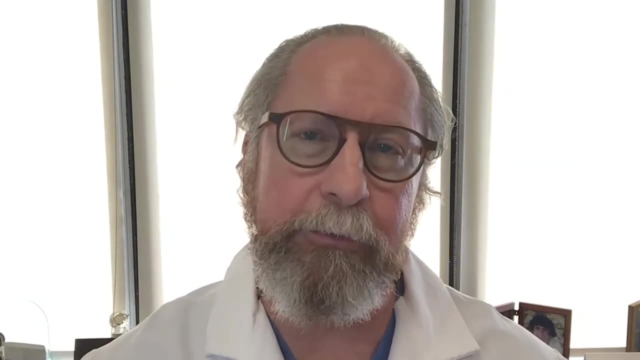 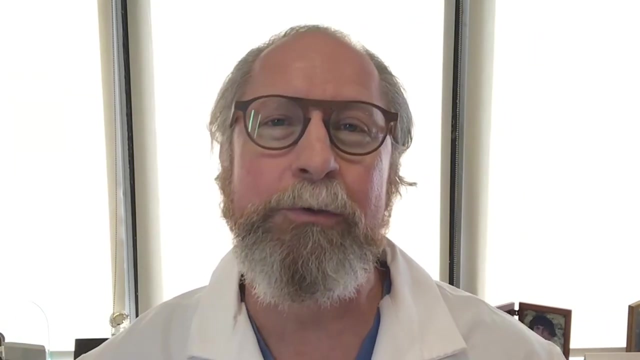 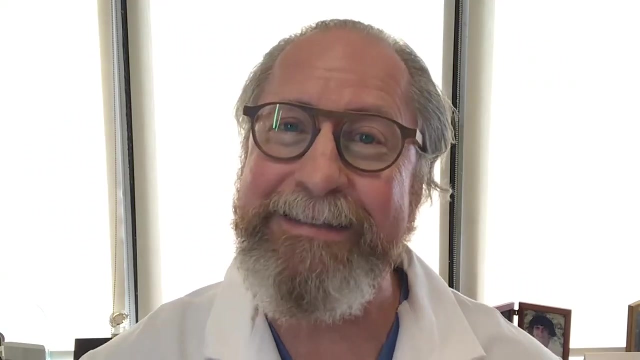 We have an apparatus, you know, in our immune system that allows us to engage a novel, you know, foreign material, whether it's a virus or foreign tissue, and develop a well-choreographed, very strong immune response. But it takes time. 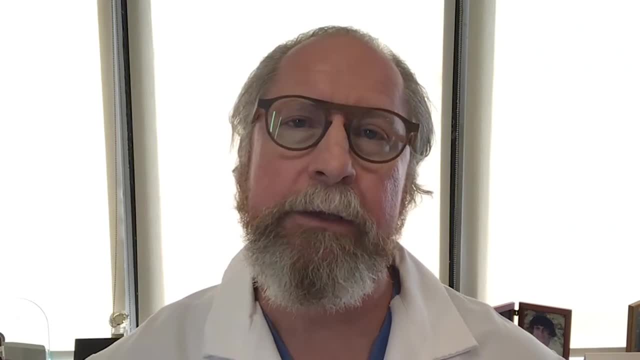 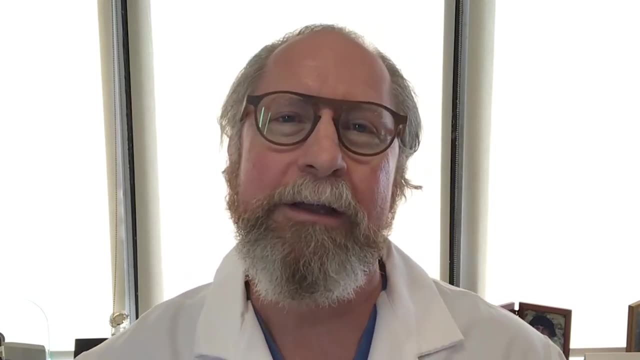 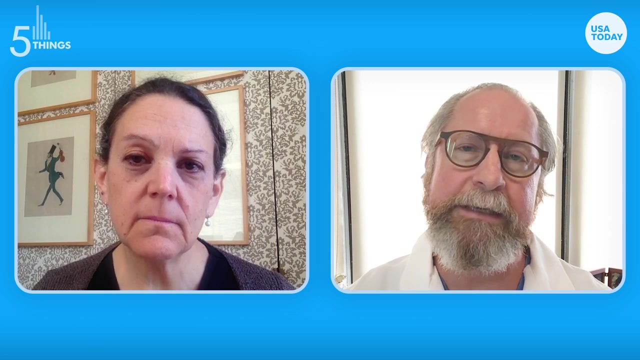 It takes somewhere between 10 to 14 days to really develop that response so that you can essentially- you know- slay the invader and get rid of that foreign material that's in your body. So the reason why we really wanted to go up to at least a month is so that we could see. that adaptive immune response fully developed. And then the second thing we were really looking at is: does the pig kidney take up all of the regular functions of the kidney, aside from just making urine and clearing toxins? And did it work? Well? it functioned great. 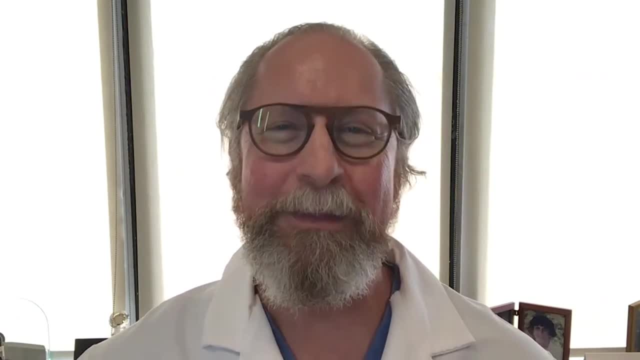 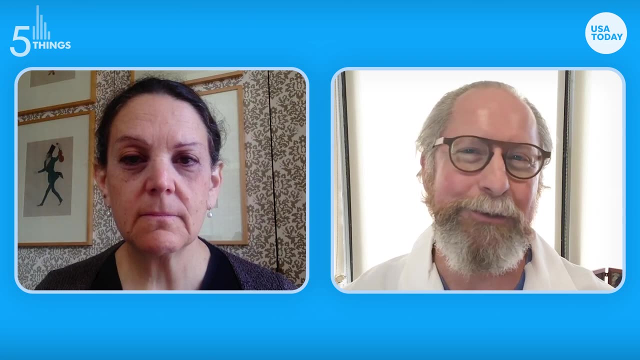 So it functioned even better than a human kidney, because actually pig kidneys have twice as much function as a human kidney. You know, the kidney was just as good, maybe even a little better. at the end of the study, at the end of the two months, 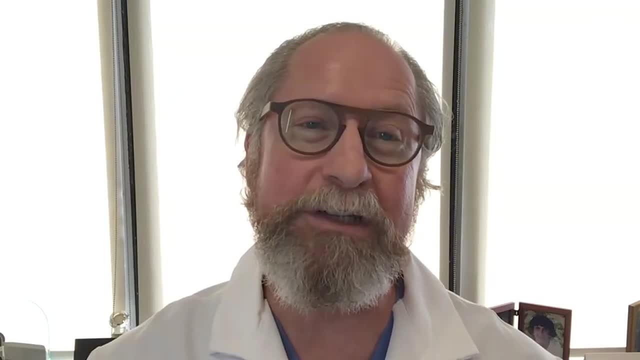 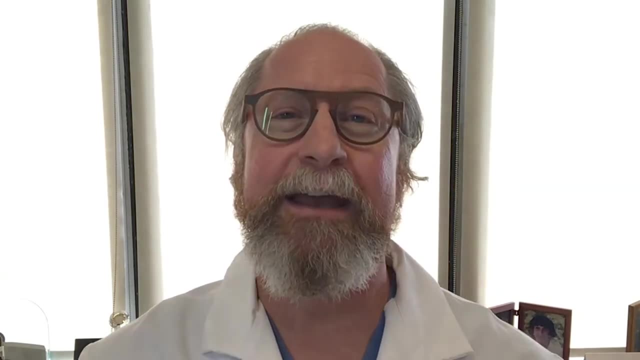 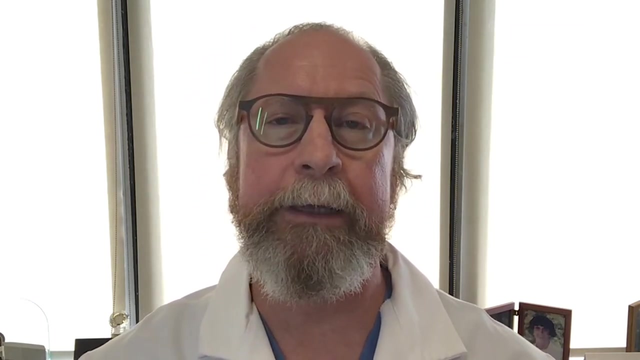 So the function was great. He did have- He did have a mild rejection, which was actually good because we could not only study it and begin to understand what rejection looks like between a human and a pig organ, but we could also treat it and use our therapeutics to try to reverse it. 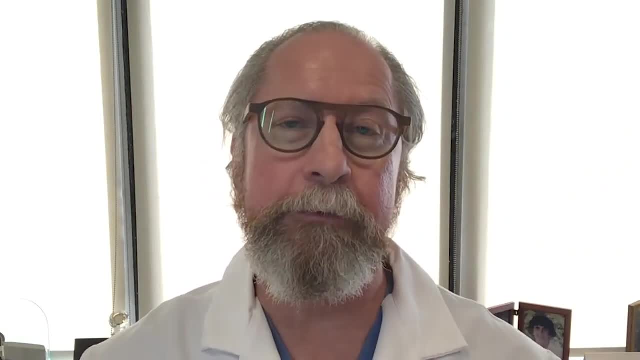 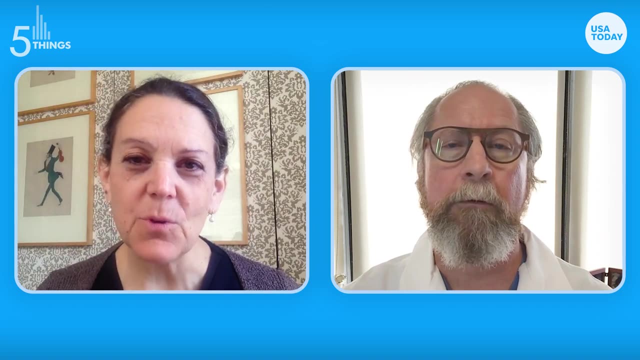 And so he had a mild rejection and it was fully reversible. And that was really important information as well. And what a next step. Yeah, Yeah, What do you think next steps look like? What do you do next in this process? 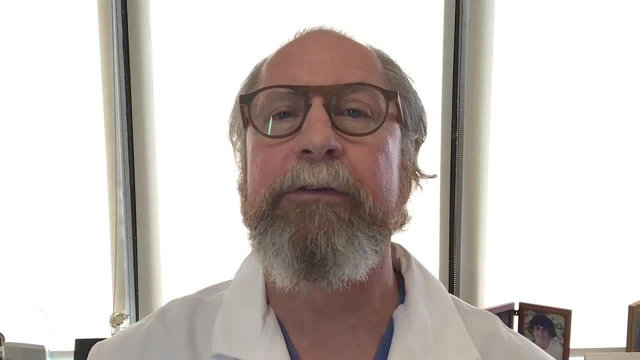 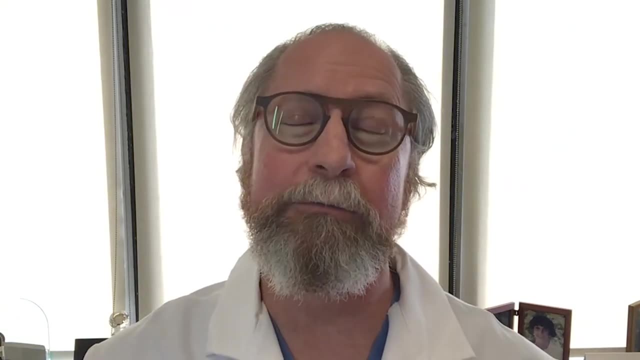 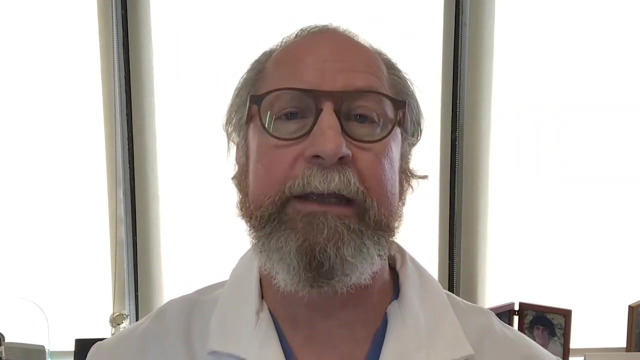 Those initial studies that we did gave us a lot of information. But this study, I think really, you know, looking at this kidney after 61 days and seeing how well it was functioning, there wasn't any protein in the urine and there wasn't. 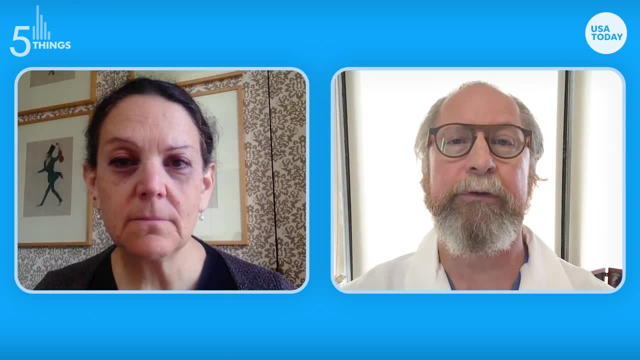 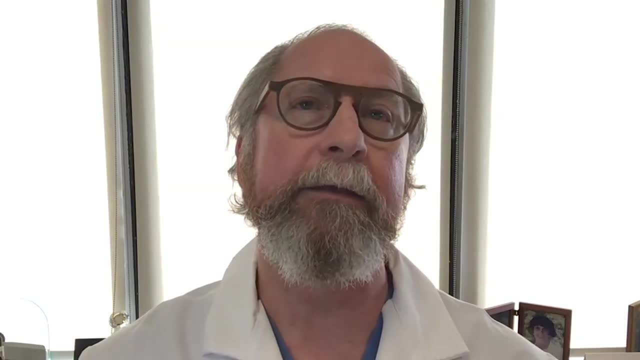 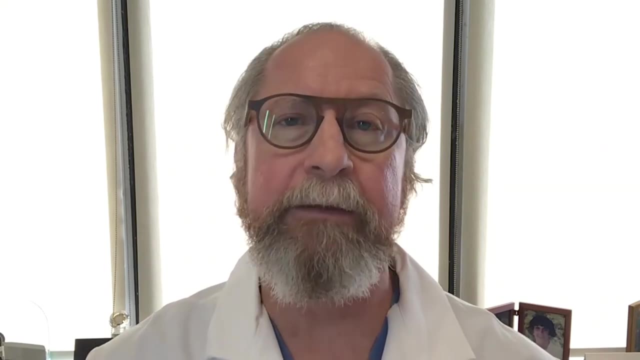 any ongoing rejection. It really looked very pristine And it was doing essentially all the things that a human kidney would do. I think this is a big jump forward And I think the FDA, once they've had an opportunity to review all the data- and we're still analyzing- 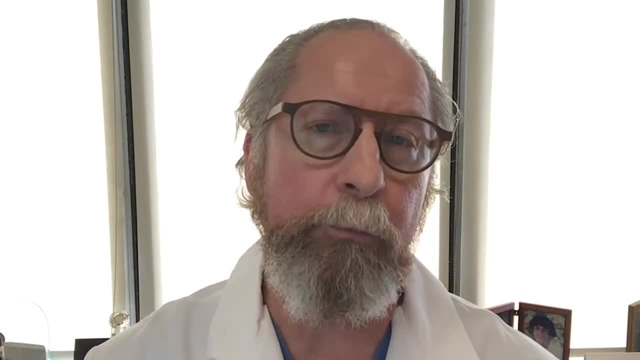 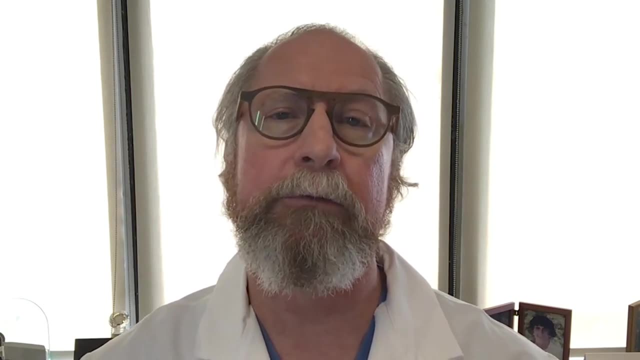 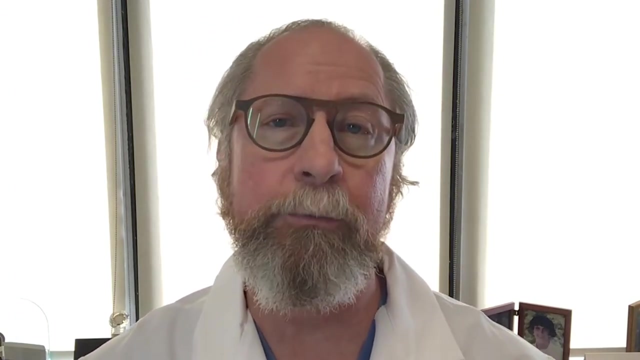 it, I think, is going to really take the work in humans and the human decedent model very seriously, Yeah, And I think it's going to accelerate us towards clinical trials. So I think you're going to start to see some living humans transplanted very soon. 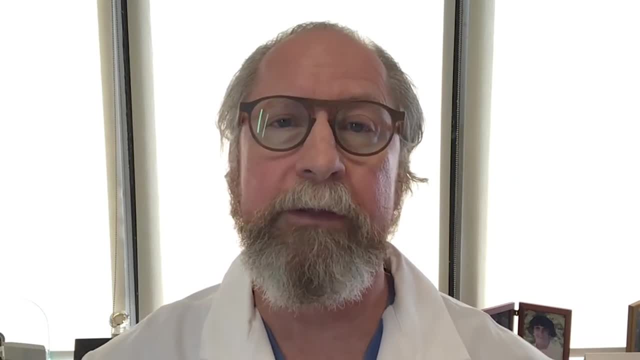 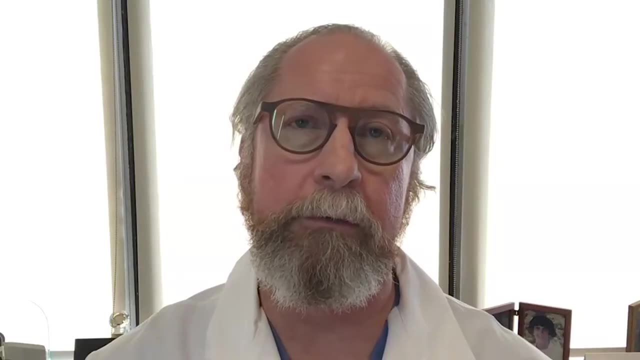 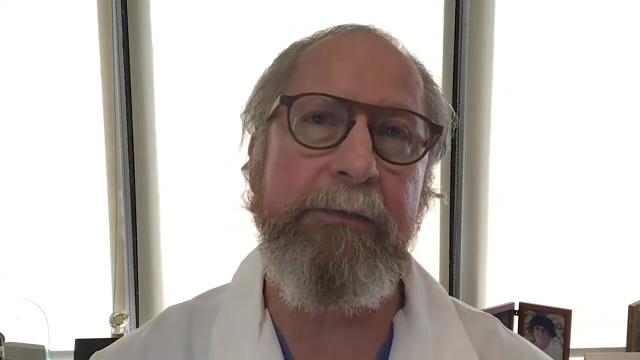 And a lot of it is going to be the result of this last study that we've just done, And how do you hope this research ultimately changes the world of transplants? The single most significant unmet need in transplantation is organ supply, And we can't even begin to estimate. We can't even begin to estimate how big that problem is, because so many people die even before they're counted on a transplant list. Only the people that we think have the best chance of survival ever even make it to a transplant list, So there's a tremendous amount of lives that are lost. 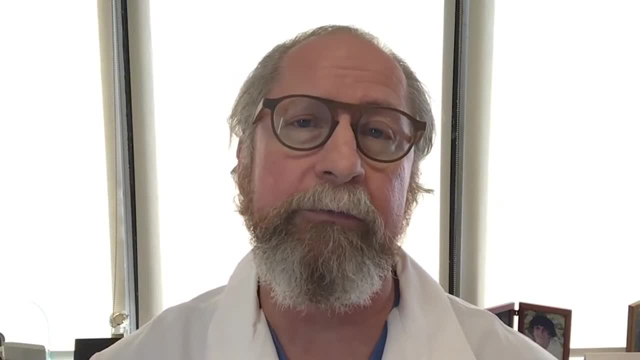 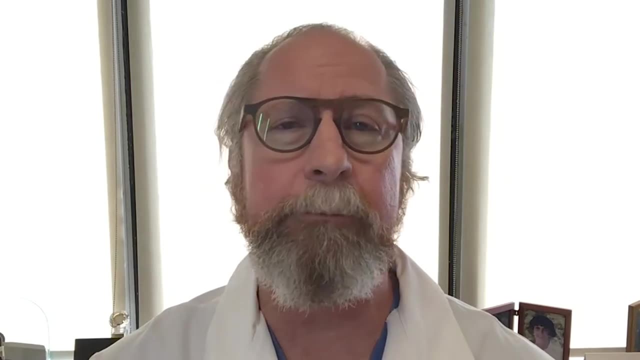 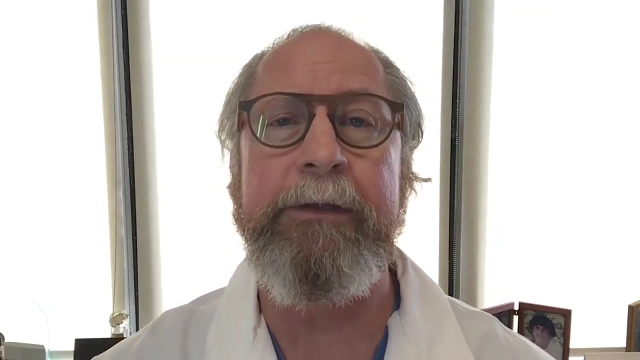 I mean myself. I had seven cardiac arrests where I had to be resuscitated. Some of them died, And some of those which required prolonged CPR that I was just very lucky to have survived before I was deemed to be sick enough to get listed for a heart transplant. And so, just to give you a sense, every year there are a million people in the United States that are newly diagnosed with heart failure. The mortality rate for heart failure over five years is 50%. Last year we were at 50%, Wow. 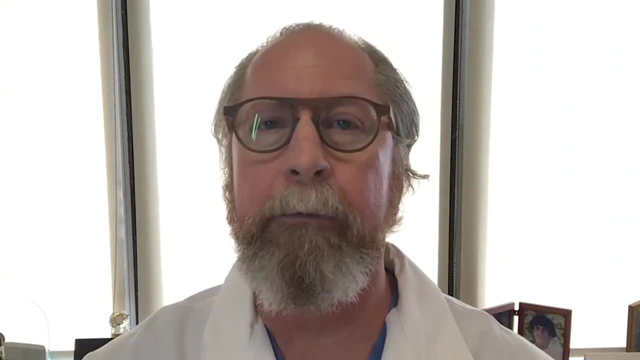 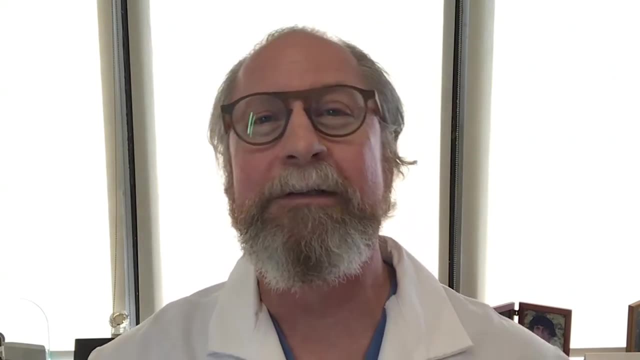 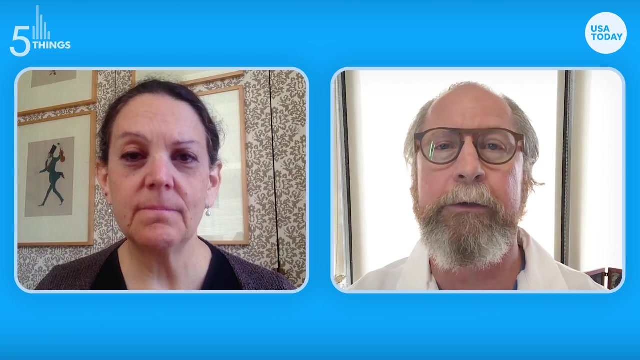 Last year we only did about 3,500, 3,600 heart transplants, So a million people with heart failure and just under 4,000 transplants. Think about that, Not even really dealing with the tip of the iceberg when it comes to organ failure in. 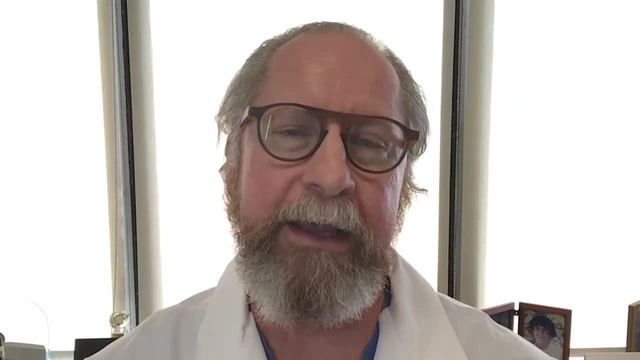 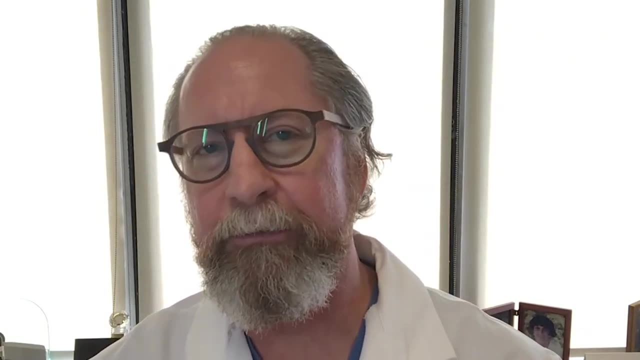 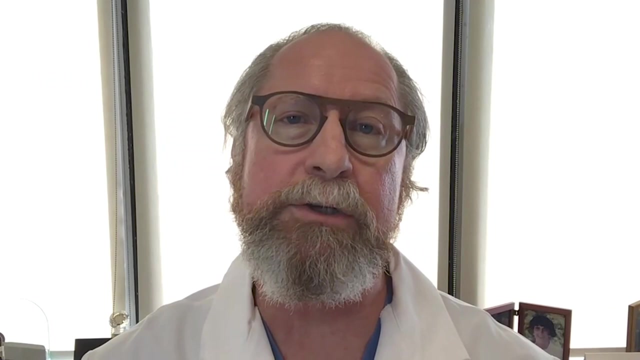 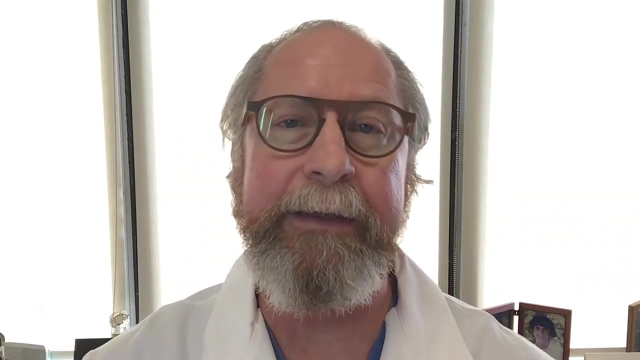 transplantation If we had an unlimited sustainable supply of organs, If we had an unlimited supply of organs that didn't require to have someone die in order for someone else to live, but we could basically, you know, whenever someone needed a transplant, at the time they needed it, rather than having them wait for years and die, you know, on